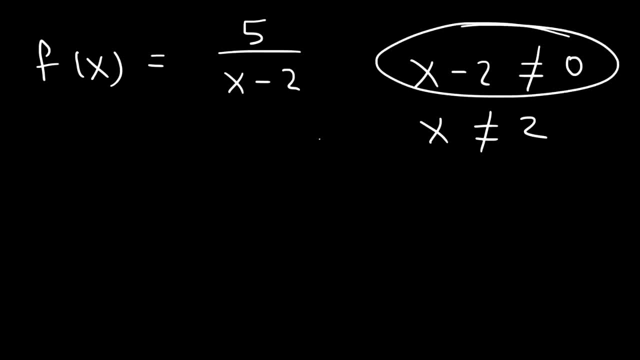 So for rational functions, set the denominator not equal to zero, and then you can find the value of x. So how do you represent this using interval notation? So if we draw a number line, x could be anything except 2.. So at 2, we're going to have an open circle. 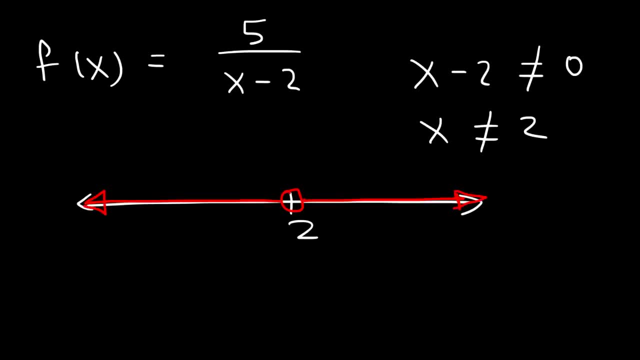 It can be greater than 2, or it can be less than 2.. All the way to the left you have negative infinity. All the way to the right, positive infinity. So for the left side, x could be anything from negative infinity to 2,, but not including. 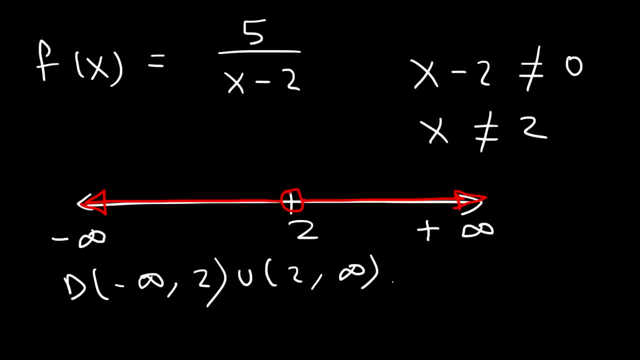 2. Or it could be anything from 2 to infinity, And so that's how you can write the, the domain, using interval notation for this example. Let's try another example. Let's say, if we have 3x minus 8, divided by x, squared minus 9x plus 20.. 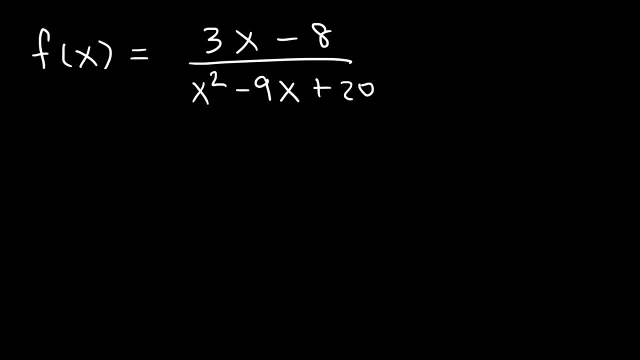 So we have another rational function, as seen by the fraction that we have. So what we need to do- just like before- and, by the way, you could try this problem if you want to- We need to set this not equal to 0.. 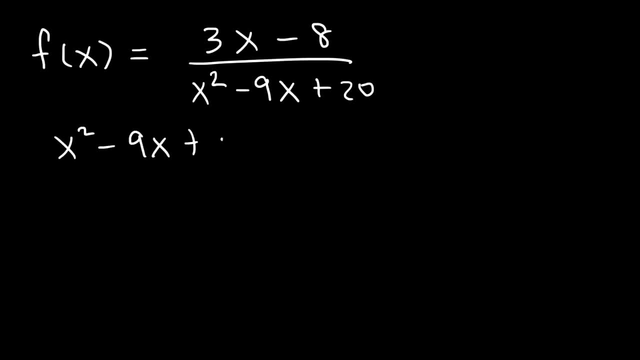 So x squared minus 9x plus 20 cannot equal 0.. So how can we find the x values that will produce a 0 in the denominator? What we need to do is we need to factor this trinomial. So what you want to do is you want to find two numbers that multiply to 20, but add to 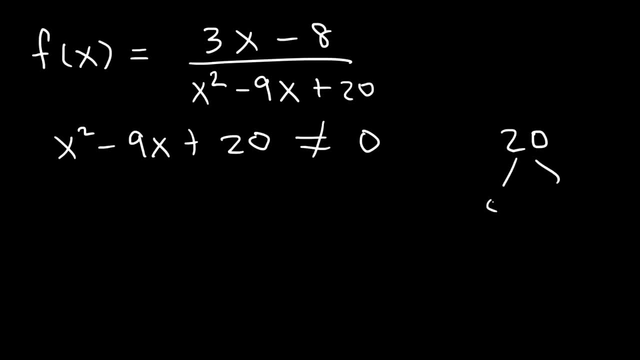 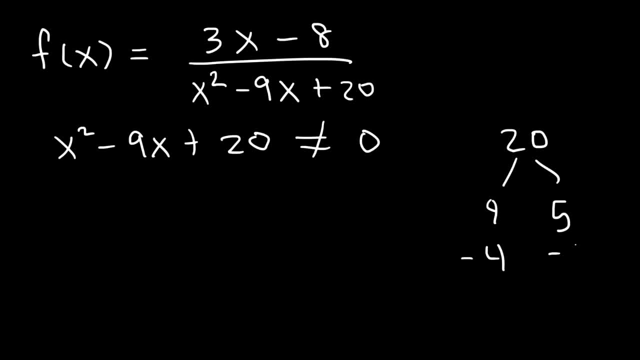 But they add up to 9, so we have to use negative 4 and negative 5., Which still multiplies to a positive 20, but add up to negative 9.. So therefore, x minus 4 times x minus 5 cannot equal 0.. 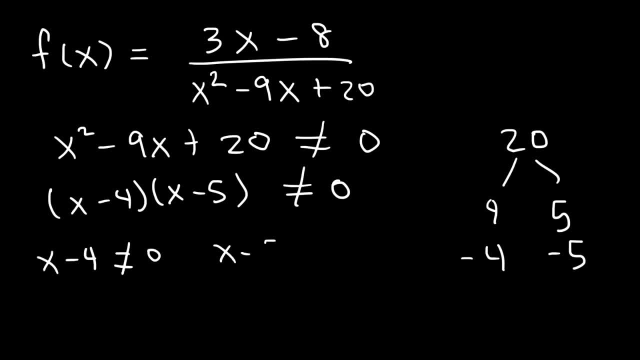 So we can say that x minus 4 cannot be 0, and x minus 5 cannot be 0.. In the first one let's add 4 to both sides, So x can't be 4, and for the second one x can't be 5.. 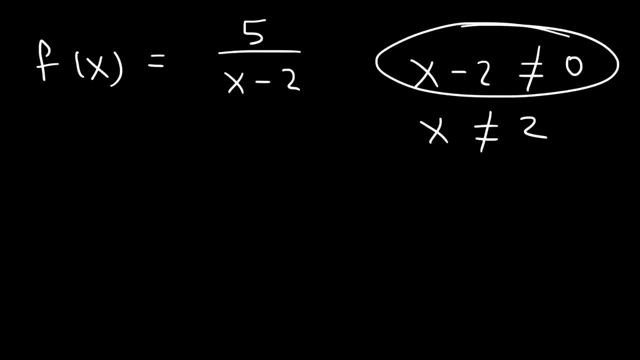 functions. set the denominator not equal to zero, and then you could find the value of x. So how do you represent this using interval notation? So if we draw a number, line, x could be anything except 2.. So at 2, we're going to have an. 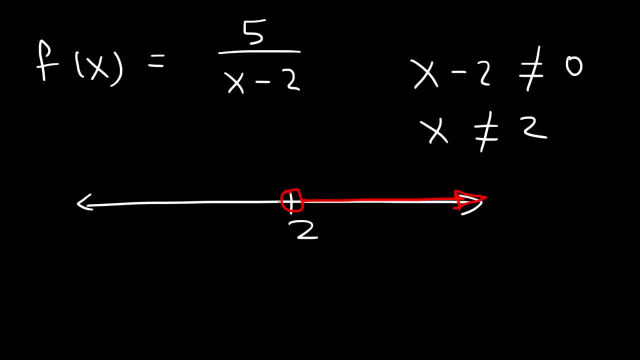 open circle. It can be greater than 2, or it can be less than 2.. All the way to the left you have negative infinity, All the way to the right, positive infinity. So for the left side, x could be anything from negative infinity to 2,, but not including 2, or it. 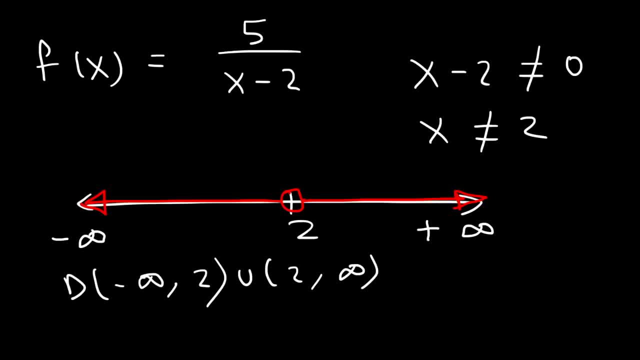 could be anything from 2 to infinity, And so that's how you can write the domain of a plane, using interval notation for this example. Let's try another example. Let's say, if we have 3x minus 8 divided by x squared minus, 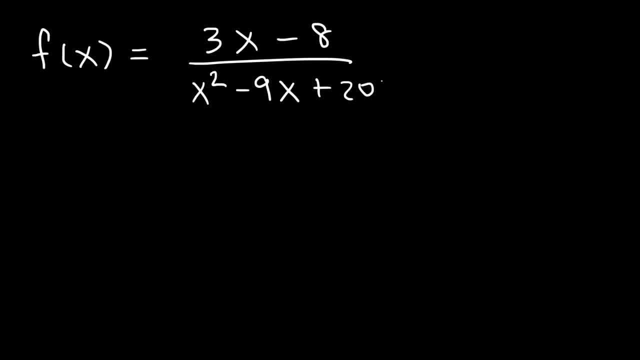 9x plus 20.. So we have another rational function, as seen by the fraction that we have. So what we need to do, just like before- and, by the way, you could try this problem if you want to- We need to set this not equal to 0.. So x squared minus 9x plus 20 cannot equal 0. So 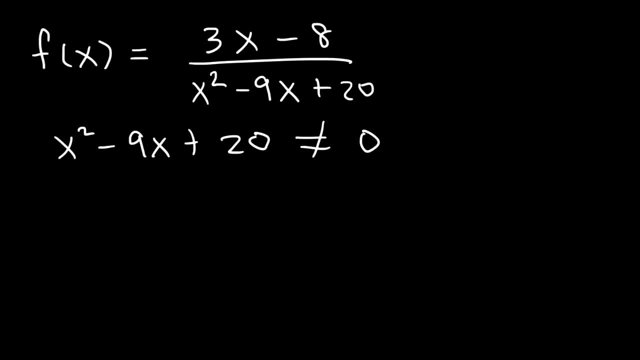 how can we find the x values that will produce a 0 in the denominator? What we need to do is we need to factor this trinomial. So what you want to do is you want to find two numbers that multiply to 20, but add to the middle coefficient negative 9.. So we know that. 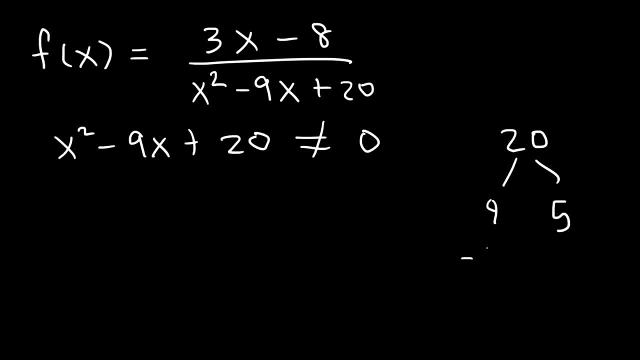 4 times 5 is 20.. But they add up to 9.. So we have to use negative 4 and negative 5,, which still multiplies to a positive 20, but add up to negative 9.. So therefore, x minus 4 times x minus 5 cannot. 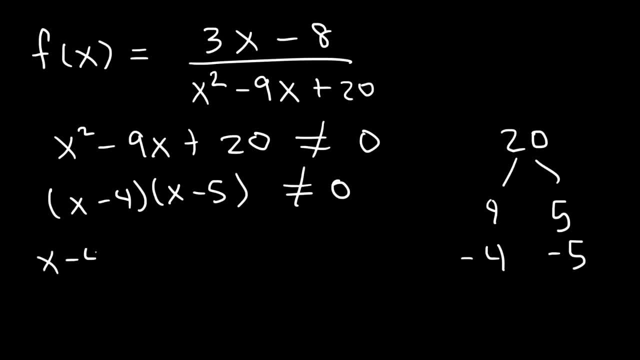 equal 0. So we could say that x minus 4 cannot be 0, and x minus 5 cannot be 0. In the first one let's add 4 to both sides, So x can't be 4.. And for the second one, x can't be. 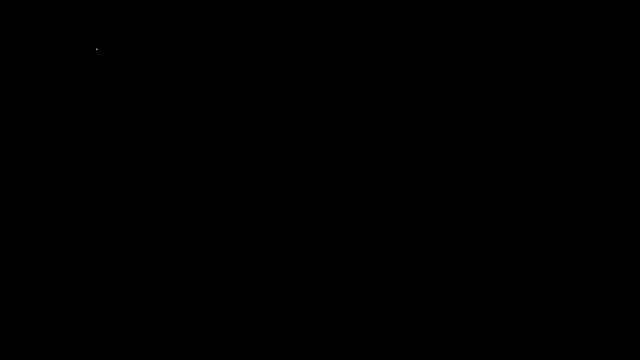 5.. Now, how do we represent this in interval notation? What I like to do is plot everything on a number line. So if x can't equal 4, I'm going to put an open circle. and it can't equal 5 either, but it can be anything else. So now lets write the domain. So from this, 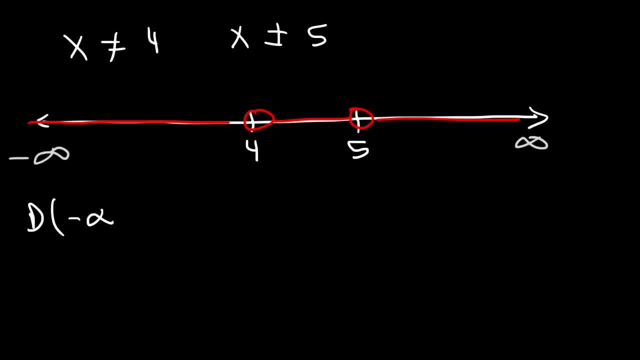 section negative infinity to 4, but it doesn't include 4. and then union. we have the second section, which goes from 4 to 5, and then union, the last section, which is 5 to infinity. so X could be anything except 4 and 5. now what about this? 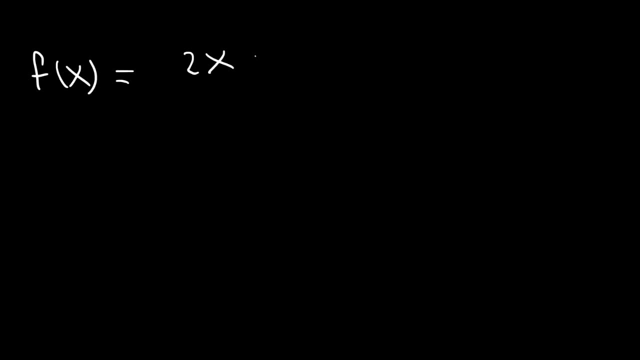 example, 2x minus 3 divided by x squared plus 4. go ahead and find the domain. so let's begin by setting x squared plus 4 not equal to 0. so if we subtract both sides by 4, we'll get this. x squared cannot equal negative 4. now this will: 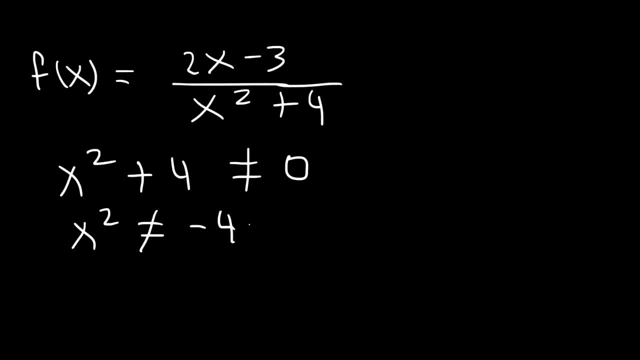 never happen. whenever you square a number, you're gonna get a positive number, not a negative number. you're gonna get a positive number, not a negative number. for example, 3 times 3 is 9 negative. 3 times negative, 3 is positive, 9, so x. 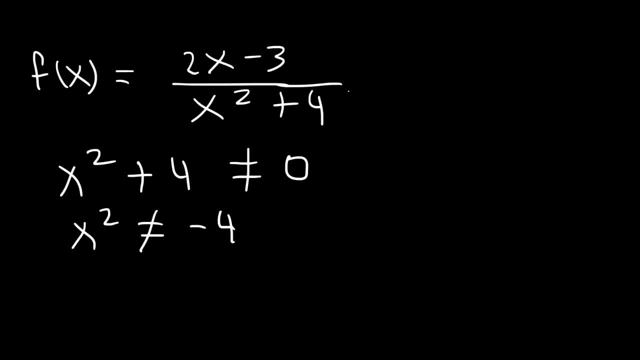 squared will never equal negative 4. so therefore, regardless of what X value you choose, the denominator will never be 0. if you plug in 2, your denominator will be 2 squared plus 4, which is 8. if you plug in negative, 2 is still gonna be 8. 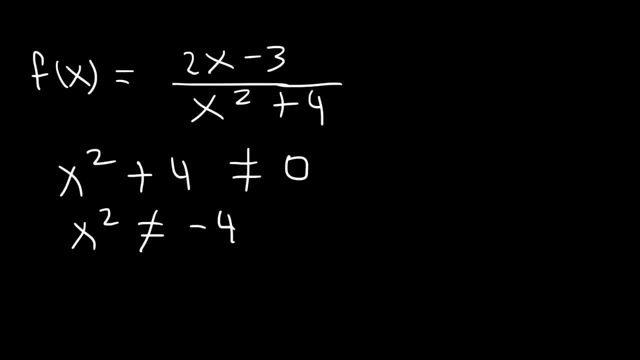 if you plug in 0 is gonna be 4. it will never equals 0 in the denominator. so therefore, for this particular rational function, it's all real numbers. the domain is from negative infinity to positive infinity. now what if you encounter a square root problem? so, for example, what is the domain of the square root of X minus 4? 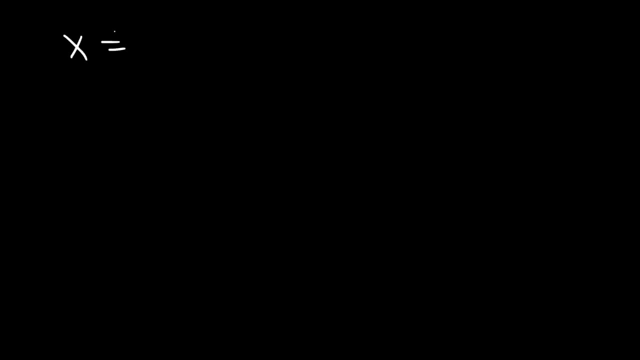 Now, how do we represent this in interval notation? What I like to do is plot everything on a number line. So if x can't equal 4, I'm going to put an open circle. and it can't equal 5 either. 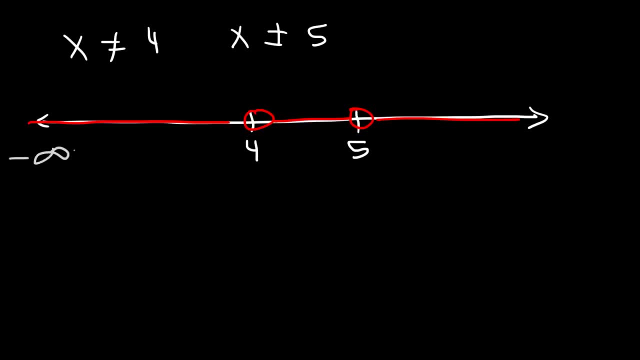 But it can be anything else. So now let's write the domain. So from this section, It's from negative infinity to 4, but it doesn't include 4.. And then union: we have the second section, which goes from 4 to 5.. 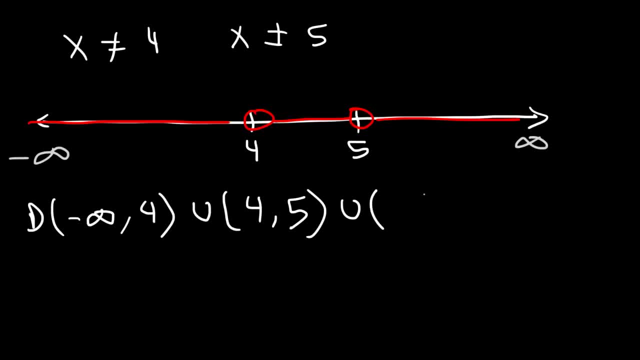 And then union the last section, which is 5 to infinity. So x can be anything except 4 and 5.. Now what about this example: 2x minus 3.. 2x minus 3.. 3 divided by x squared plus 4.. 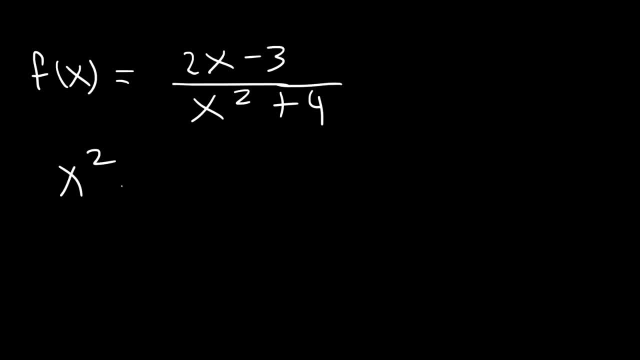 Go ahead and find the domain. So let's begin by setting x squared plus 4 not equal to 0. So if we subtract both sides by 4, we'll get this: x squared cannot equal negative 4.. Now, this will never happen. 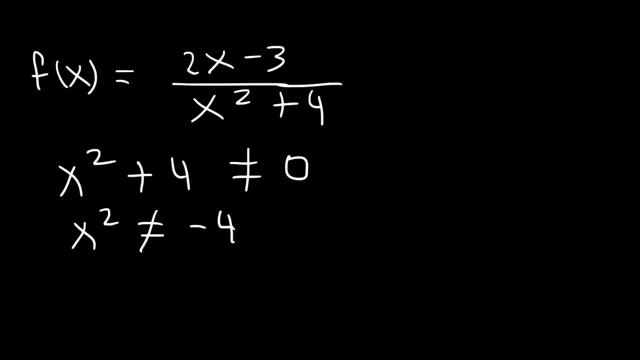 Whenever you square a number, you're going to get a positive number, not a negative number. For example, 3 times 3 is 9.. 3 times negative, 3 is positive, 9.. So x squared will never equal negative 4.. 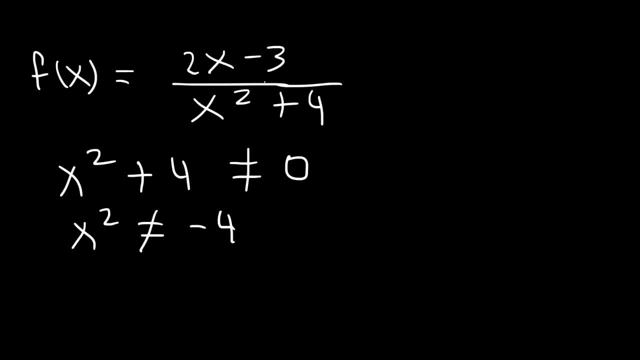 So, therefore, regardless of what x value you choose, the denominator will never be 0.. If you plug in 2, your denominator will be 2 squared plus 4, which is 8.. If you plug in negative 2, it's still going to be 8.. 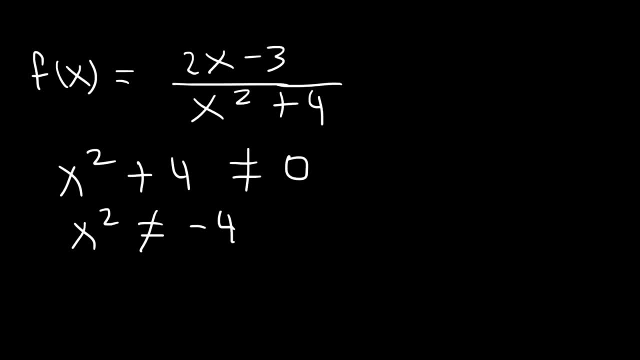 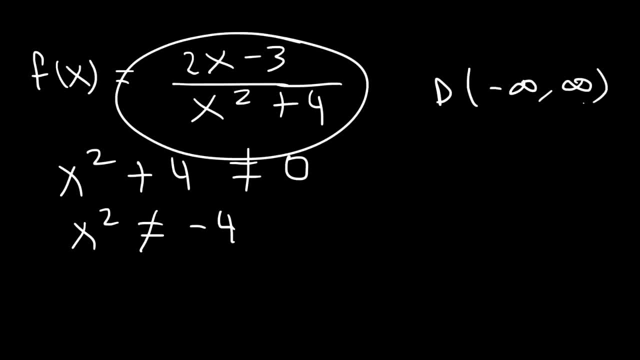 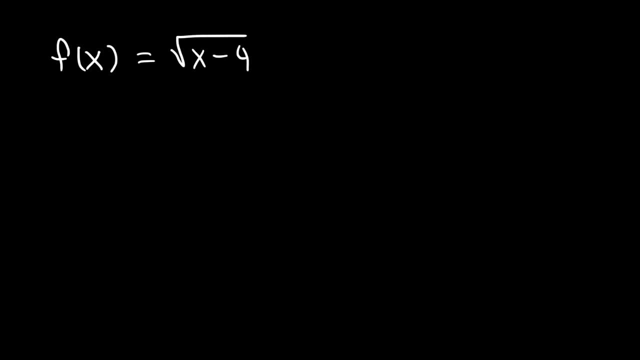 how can we find the answer now for square roots or any radical where the index numbers even you cannot have a negative number on the inside. if it's odd, it could be anything. it's R, more numbers. but for even radicals, or radicals with even index numbers, you have to set the inside greater than or 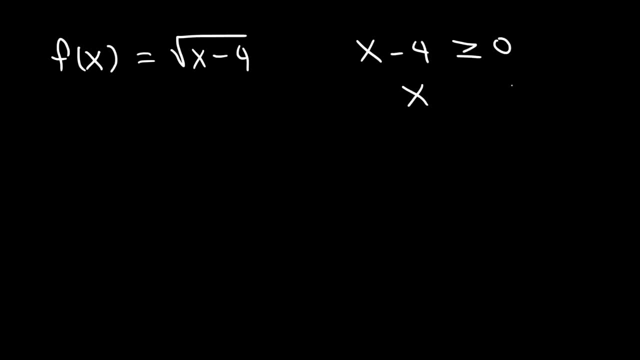 equal to 0. it can't be negative. so for this one, all we need to do is add 4 to both sides, so X is equal to or greater than 4. to represent that with a number line, we're gonna have a closed circle this time, so it could be equal to: or. 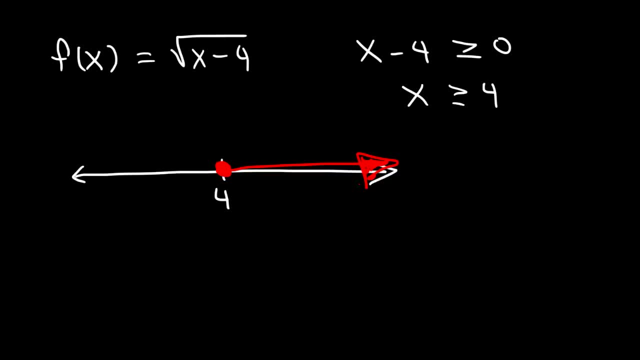 greater than so we're gonna shade to the right. so, to the right, we have positive infinity, so the domain is going to be from 4 to infinity. since it includes 4, we need to use a bracket in this case. now, what about a problem that looks like this: the square root of x squared plus: 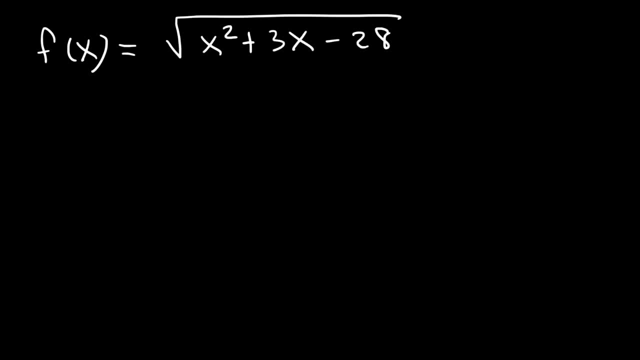 3x minus 28. how can we find the domain of this function? so, just like before, we're going to set the inside of the square root function equal to or greater than 0. now we need to factor. so let's find two numbers that multiply to negative 28. but 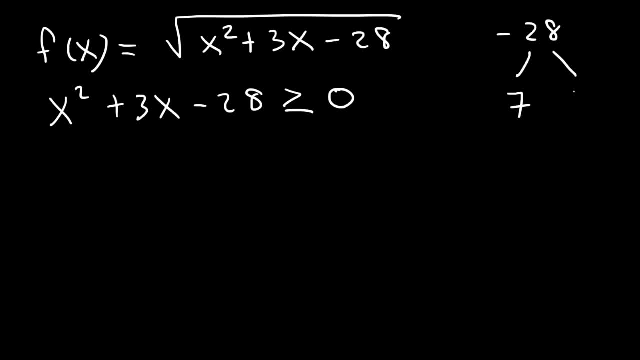 that, add to 3, so we have 7 and 4. now I need to add up to positive 3. so we're going to use positive 7 and negative 4. 7 plus negative 4 is positive 3 and 7 times negative. 4 is negative 28.. So it's a factor. it's going to be x minus 4 times x plus 7.. 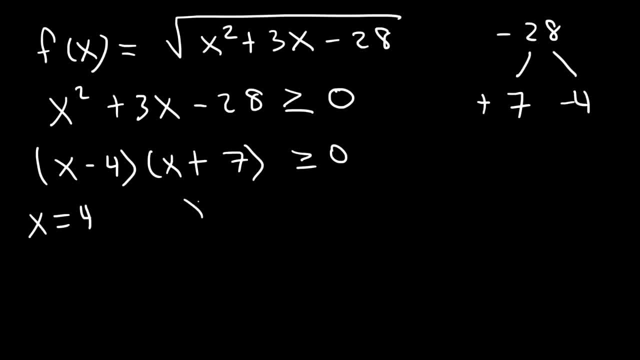 So x can equal 4 and x can equal negative 7.. Now what I'm going to do is make a number line with these two values. Now, negative 7 and 4 are included, so let's put a closed circle. Now for this type of problem, we need to be careful. We need to find out which of 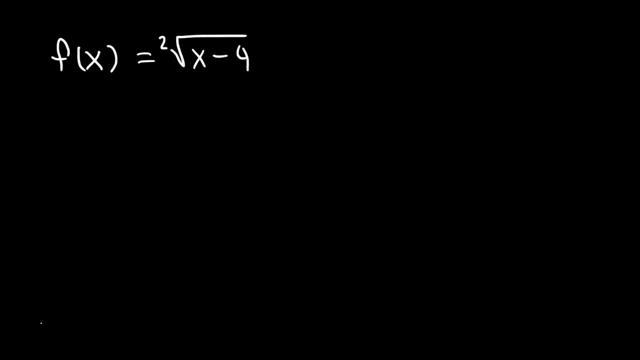 Now for square roots or any radical where the index number is even. you cannot have a negative number on the inside. If it's odd, it could be anything. It's all real numbers. But for even radicals, or radicals with even index numbers, 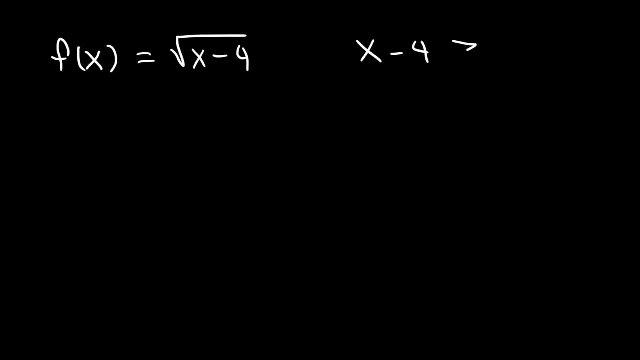 you have to set the inside greater than or equal to 0. It can't be negative. So for this one, all we need to do is add 4 to both sides, So x is equal to or greater than 4.. To represent that with a number line we're going to have a closed circle this time. 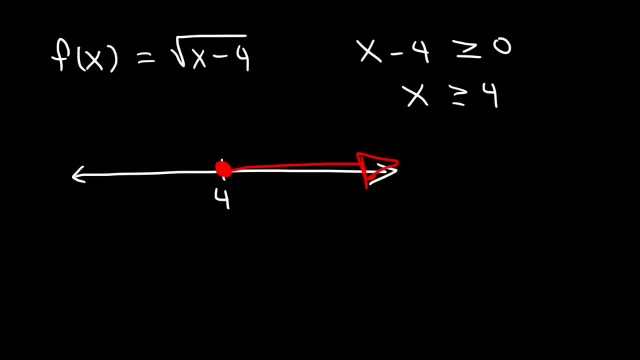 So it could be equal to or greater than so. we're going to shade to the right. So to the right, we have positive infinity, So the domain is going to be from 4 to infinity. Since it includes 4, we need to use a bracket in this case. 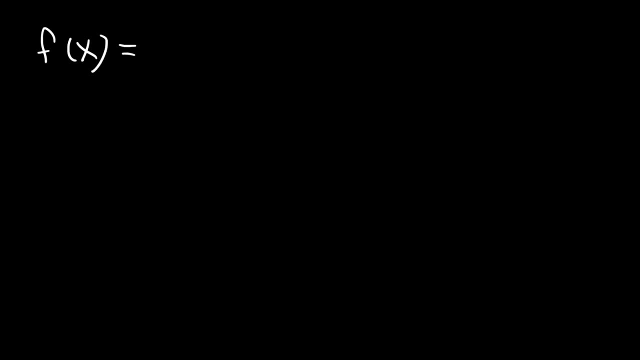 Now, what about a problem that looks like this: The square root of x, squared plus 3x minus 28.. How can we find the domain of this function? So, just like before, we're going to set the inside of the square root function equal to or greater than 0.. 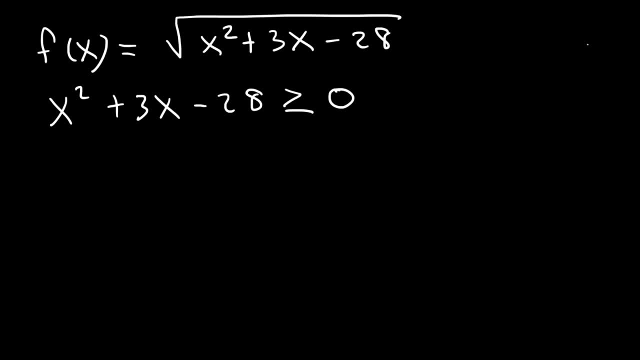 Now we need to factor. So let's find two numbers that multiply to negative 28, but that add to 3. So we have 7 and 4.. Now I need to add up to positive 3, so we're going to use positive 7 and negative 4.. 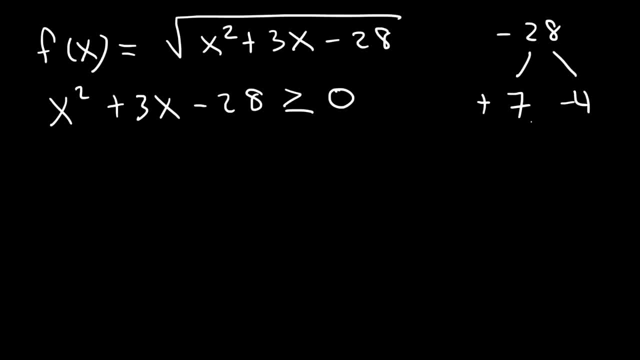 7 plus negative. 4 is positive 3. And 7 times negative 4 is negative 28. So to factor, it's going to be x minus 4 times x plus 7. So x can equal 4 and x can equal negative 7.. 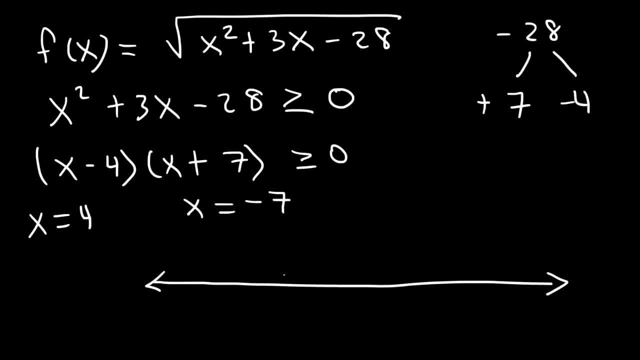 Now what I'm going to do is make a number line with these two values. Now, negative 7 and 4 are included, So Let's put a closed circle Now for this type of problem. we need to be careful. 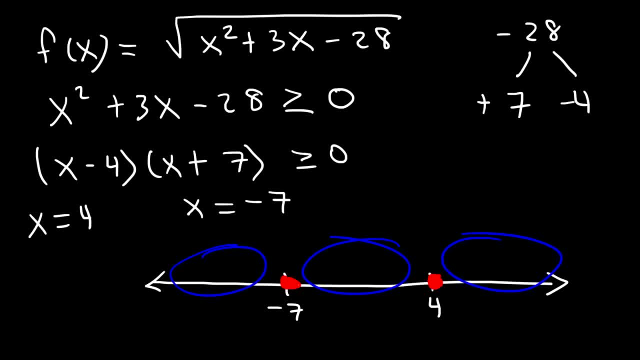 We need to find out which of these three regions will work. So we need to check the signs, We need to see which one is positive and which one is negative. So let's check this region first. If we pick a number that's greater than 4, like 5,, and if we plug it into this expression, 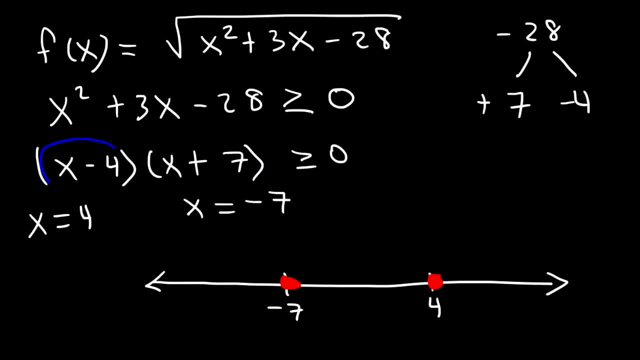 will it be positive or negative? Well, if we plug in 5,, 5 minus 4 is a positive number And 5 plus 7 is a positive number. When you multiply two positive numbers together, you're going to get a positive result. 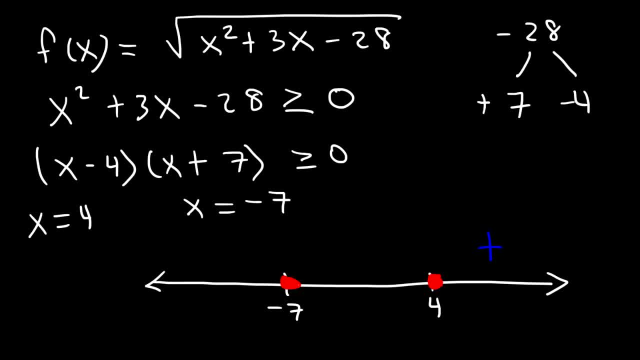 Now, if we pick a number between negative 7 and 4, let's say 0, and plug it in: 0 minus 4 is negative. 0 plus 7 is positive. A negative number times a positive number is a negative number. 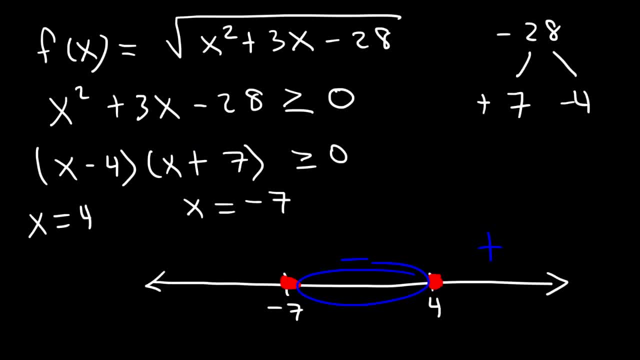 So if we choose any number in this region, it's going to give us a negative result. Now, if we choose a number that's less than negative 7, like negative 8, negative 8 minus 4 is negative. Negative 8 plus 7 is negative. 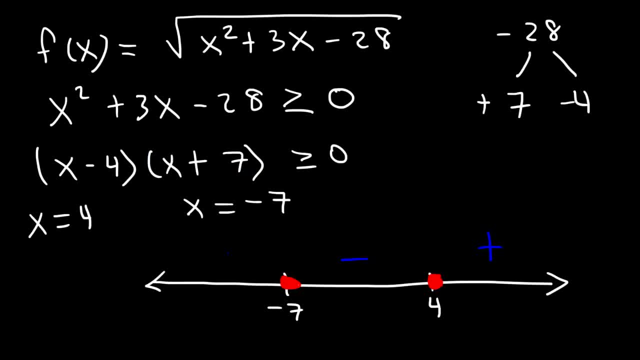 When you multiply two negative numbers, you're going to get a positive result. Now, we can't have any negative numbers inside the square root symbol, So therefore we're not going to have any solution in that region. So therefore we should only: 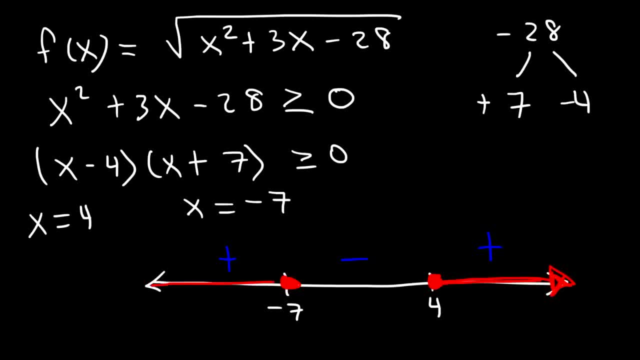 Let's shade the positive regions. So now we can have the answer. So x can be less than negative 7,, that's, to the left, less than or equal to negative 7, or x can be equal to or greater than 4.. 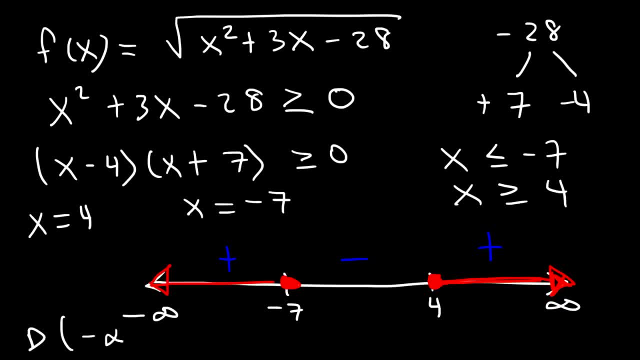 Now to represent this using interval notation. it's going to be from negative infinity to negative 7, and then union: We're going to start. We're going to start back up at 4 to infinity, And we need to use brackets at 7, I mean negative 7 and 4,. 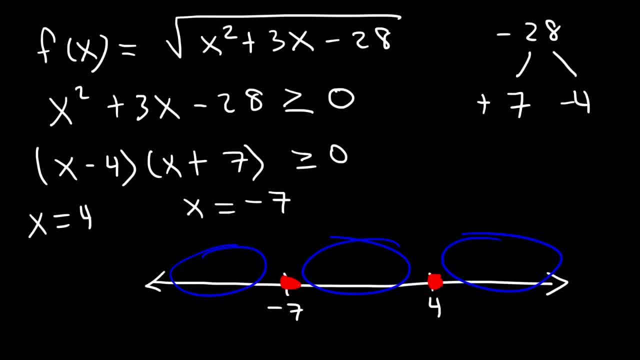 these three regions will work. So we need to check the signs, We need to see which one is positive and which one is negative. So let's check this region first. If we pick a number that's greater than 4, like 5, and if we plug it into this expression, 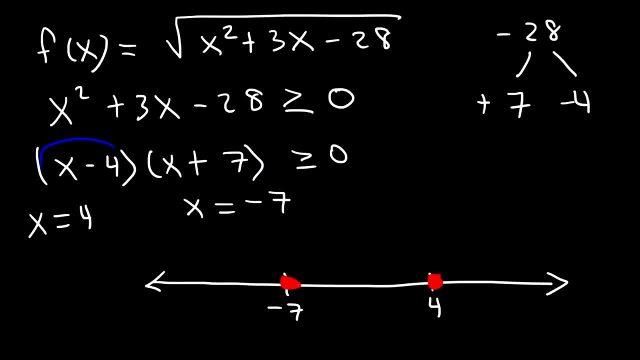 will it be positive or negative? Well, if we plug in 5,, 5 minus 4 is a positive number and 5 plus 7 is a positive number. When you multiply two positive numbers together, you're going to get a positive result. Now, if we pick a number between negative 7 and 4, let's 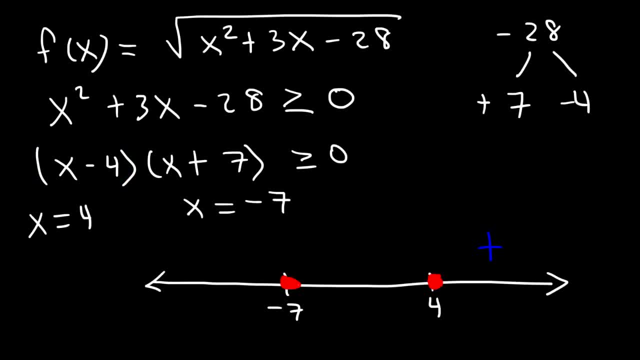 say 0, and plug it in: 0 minus 4 is negative. 0 plus 7 is positive. A negative number times a positive number is a negative number. So if we choose any number in this region, it's going to give us a negative result. Now, if 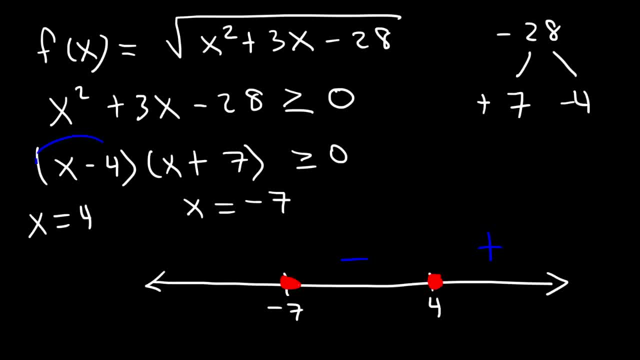 we choose a number that's less than negative 7, like negative 8, negative 8 minus 4 is negative. Negative 8 plus 7 is negative. When you multiply two negative numbers, you're going to get a positive result. 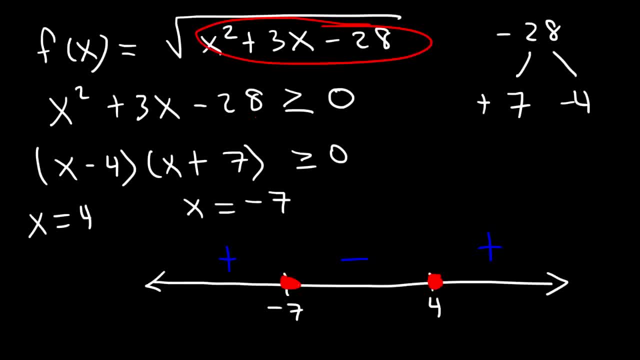 Now we can't have any negative numbers inside the square root symbol. So therefore we're not going to have any solution in that region. So therefore we should only shade the positive regions. So now we can have the answer. So x can be less than negative 7, that's to the left. 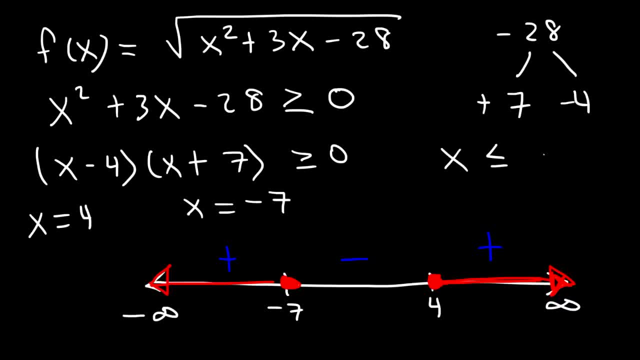 less than or equal to negative 7.. Or x can be equal to or greater than 4.. Now to represent this using interval notation, it's going to be from negative infinity to negative 7, and then union we're going to. 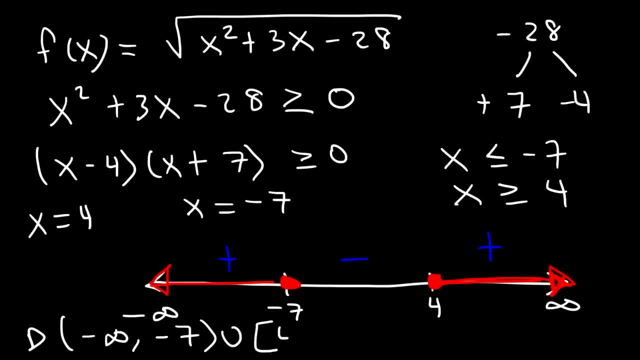 start back up at 4 to infinity, And we need to use brackets at 7, I mean negative 7 and 4, because it includes those two points. So we have a closed circle there. So that's how you could find the domain of this type of formula. 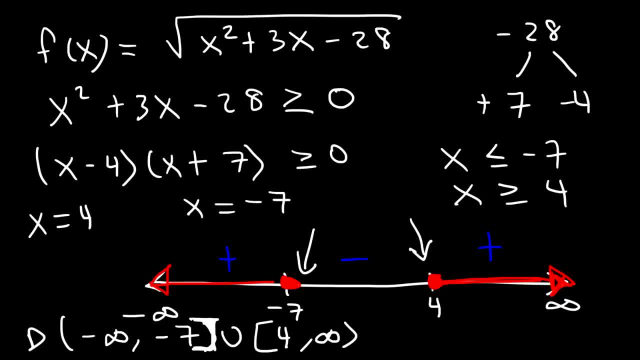 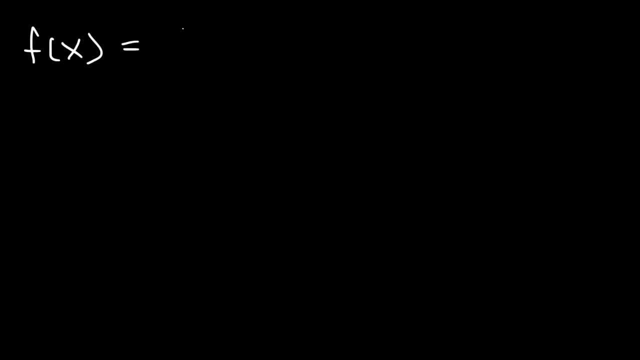 because it includes those two points. We have a closed circle there. So that's how you can find the domain of this type of function. Now, sometimes you may have a fraction with a square root. So what do you do If the square root is in the denominator of the fraction? 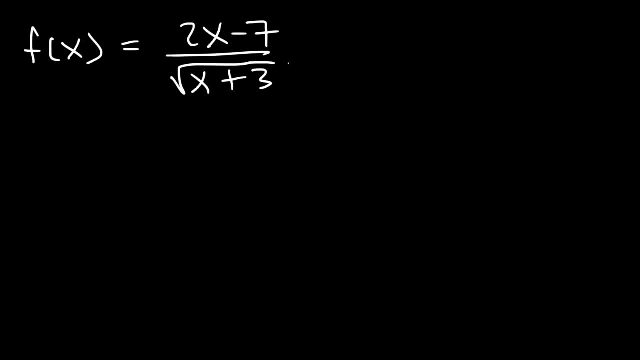 Now, if the square root was not in the denominator, we would set the inside equal to and greater than 0. But we can't have a 0 in the bottom of a fraction, So this time we can only set the inside just greater than 0.. 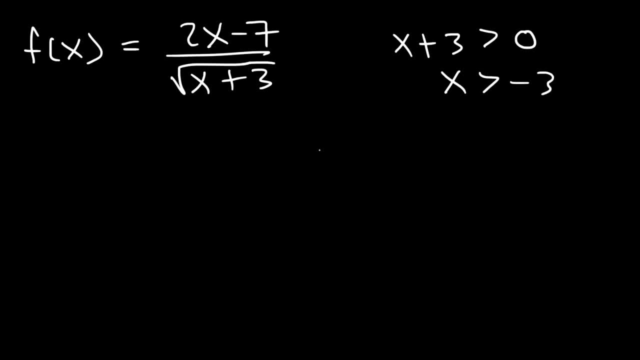 So x has to be greater than negative 3.. So the domain is simply going to be from negative 3 to infinity, But not including negative 3.. Now let's consider another example. So we're going to have a fraction again. 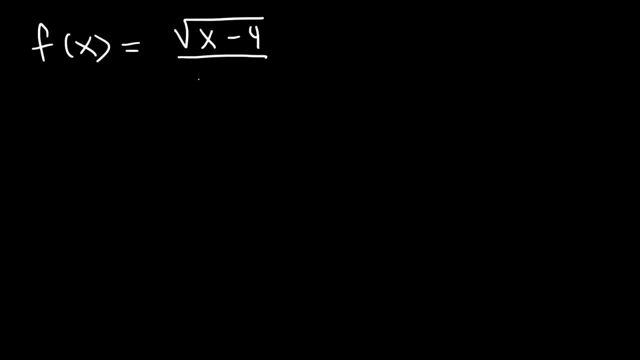 but with a square root in the numerator. What do you think the domain for this function is going to be? Now, if you have a square root in the numerator, you need to set the inside equal to or greater than 0.. So x is equal to and greater than 0.. 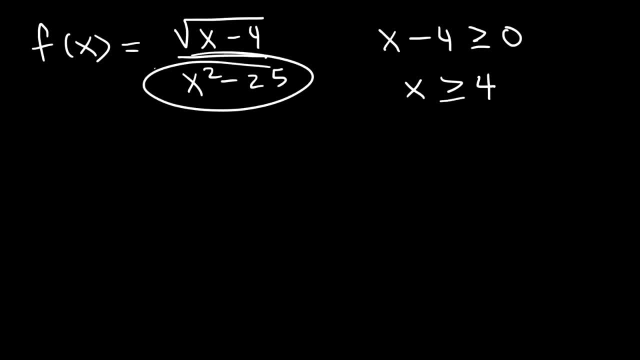 Now we know that in a denominator we can't have a 0. So we're going to set it equal or not equal to 0. And we can factor it. So this is going to be x plus 5 times x minus 5,. 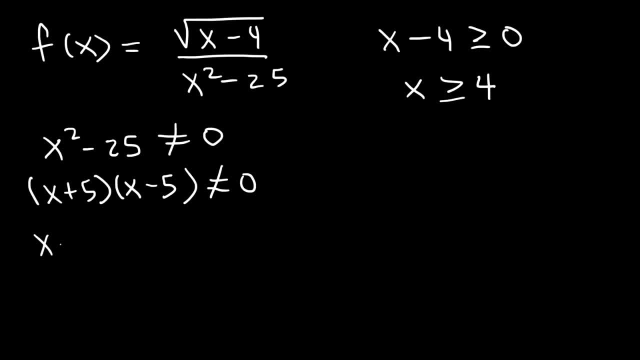 using the difference of squares method. So x cannot equal negative 5, and it can't equal 5.. So now let's make a number line. So we have negative 5, 4. And 5.. So we're going to have an open circle at negative 5 and 5.. 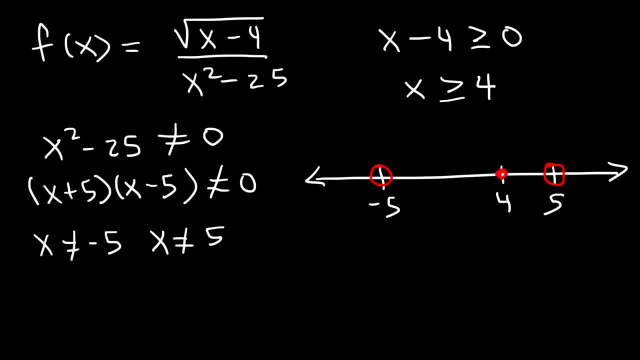 And then x is equal to or greater than 4.. So we're going to have a closed circle at 4 and shade to the right. So there's nothing really to write here, because x is not going to equal to anything less than 4.. 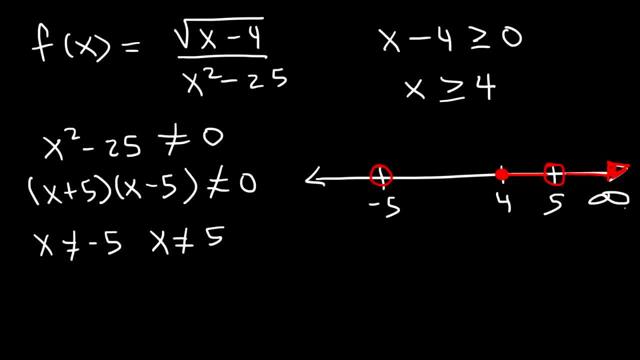 It equals everything greater than 4, including 4, but just not 5.. So how do we represent that in interval notation? So this is the first part. So we're going to start with 4 using brackets and stop at 5 using parentheses. 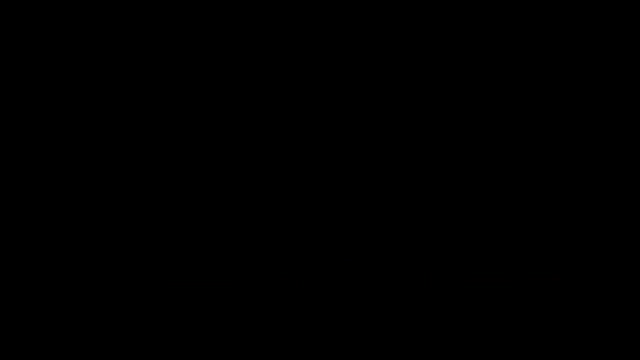 Congratulations. Subtitles by the Amaraorg community function. Now, sometimes you may have a fraction with a square root. So what do you do if the square root is in the denominator of the fraction? Now, if the square root was not in the denominator, we would set the inside equal to and. 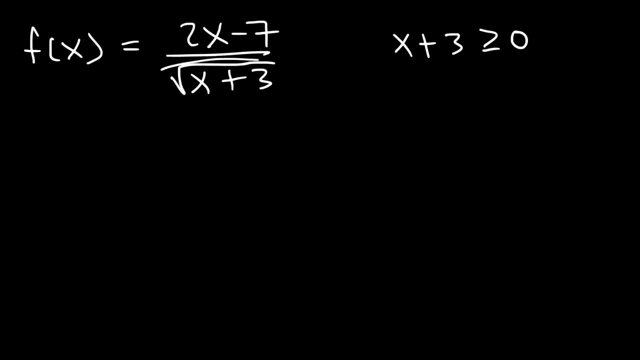 greater than 0. But we can't have a 0 in the bottom of a fraction, so this time we can only set the inside just greater than 0. So x has to be greater than negative 3.. So the domain is simply going to be from negative 3 to infinity. but 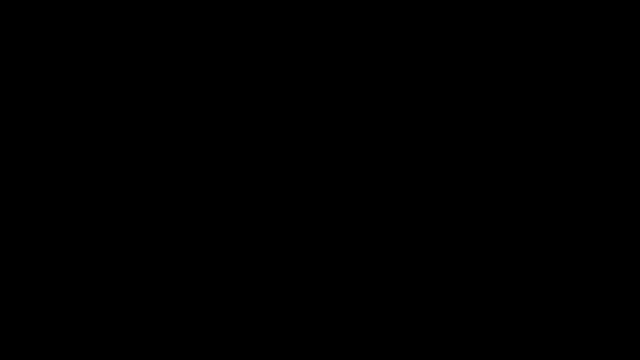 not including negative 3.. Now let's consider another example. So we're going to have a fraction again, but with a square root in the numerator. What do you think the domain for this function is going to be? Now, if you have a square root in the numerator, you need to set the inside. 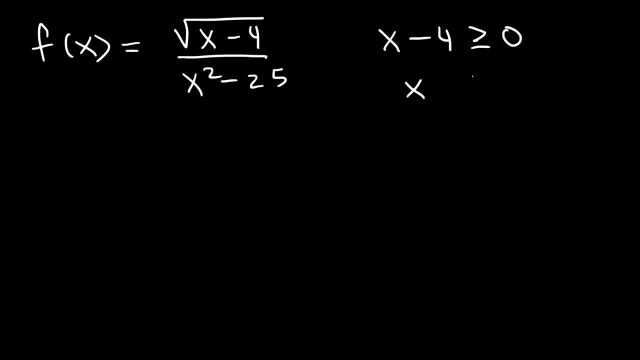 equal to or greater than 0. So x is equal to and greater than 4.. Now we know that in a denominator we can't have a 0. So we're going to set it equal or not equal to 0. And we could factor it. So this is going to be x plus 5 times x minus 5,. 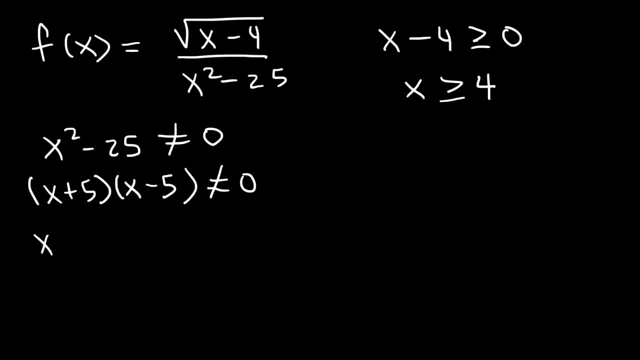 using the difference of squares method. So x cannot equal negative 5, and it can't equal 5.. So now let's make a number line. So we have negative 5,, 4, and 5.. So we're going to have an open circle at. 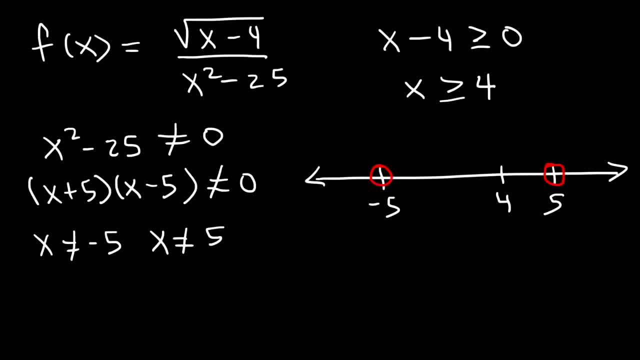 negative 5 and 5.. And then x is equal to or greater than 4.. So we're going to have a closed circle at 4 and shade to the right. So there's nothing really to write here, because x is not going to equal to anything. 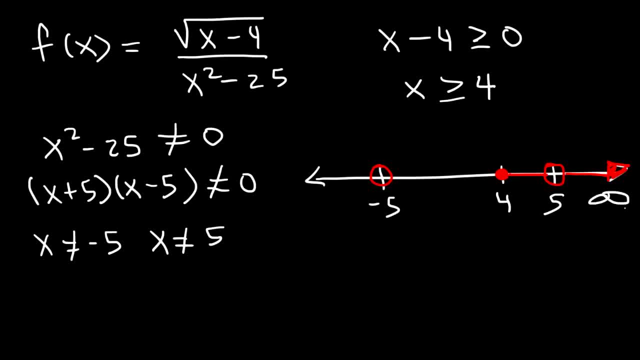 It equals everything greater than 4, including 4, but just not 5.. So how do we represent that in interval notation? So this is the first part. So we're going to start with 4 using brackets and stop at 5 using parentheses, since it does not. 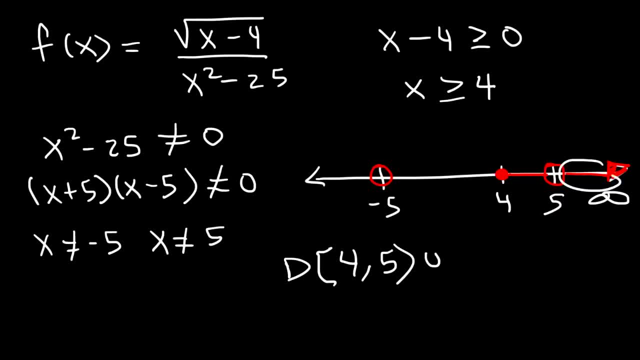 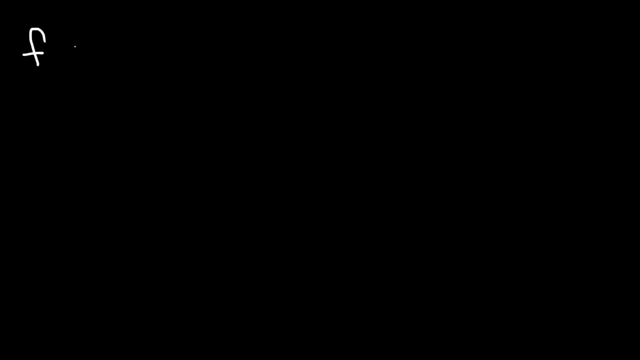 since it does not include 5.. And then union, for the second part, is going to go from 5 to infinity. So that's how you can represent the answer, using interval notation. Now, what would you do if you have a fraction that contains a square root? 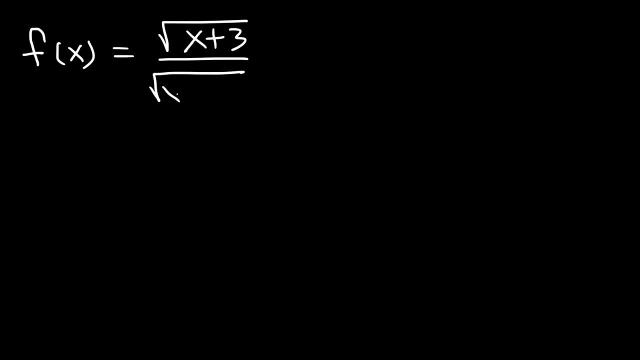 in the numerator and also in the denominator. Try this. So let's focus on the numerator. We know that x plus 3 is equal to or greater than 0, which means x is greater than or equal to negative 3.. So if we plot that on our number line, 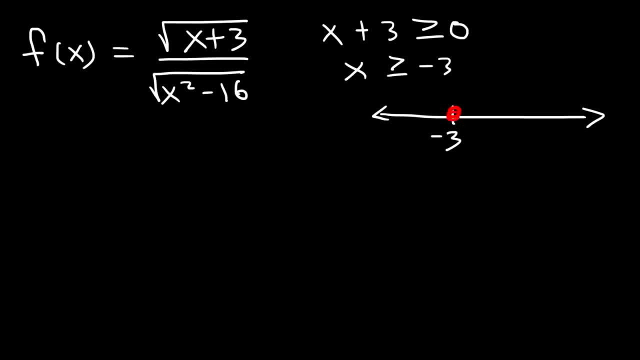 this is what we're going to have. So it's from negative 3 to infinity. Now let's focus on the square root in the bottom. So we know that x squared minus 16 has to be only greater than 0, but not equal to it, because if it's on the bottom it can't be 0.. 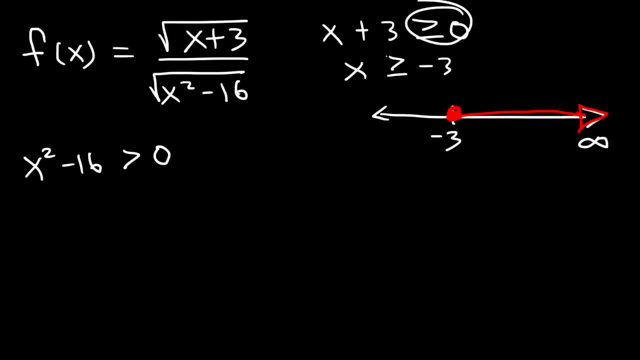 So if you have a square root on the top, you set it equal to and greater than 0. If it's on the bottom, simply just greater than 0. So what we need to do first is factor this expression. It's going to be x plus 4 and x minus 4.. 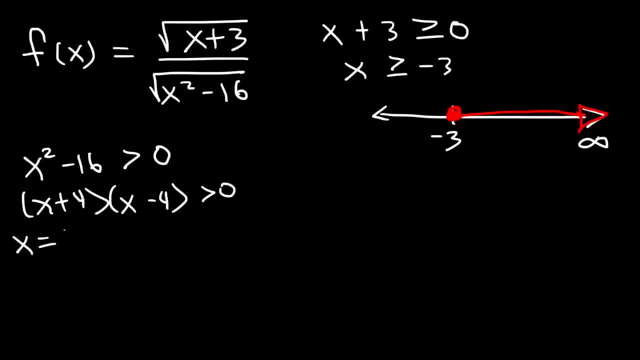 So x can't be negative 4, and x can't be 4.. But it can be equal to values in between. So we're going to make a second number line. Now, the reason why it can't equal it is because we don't have the underlined symbol. 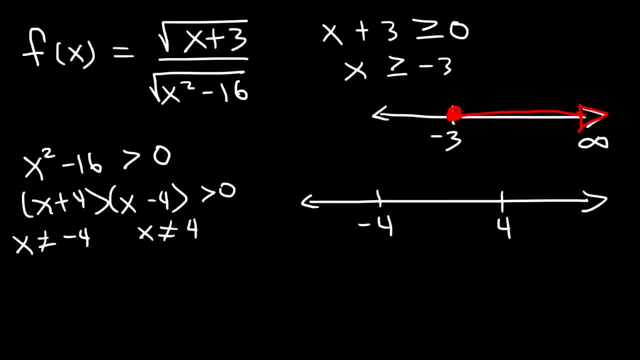 It's only greater than 0, but not equal to 0.. So let's start with an open circle at negative 4 and 4.. Now, whenever you have like two circles on a number line due to a square root function, 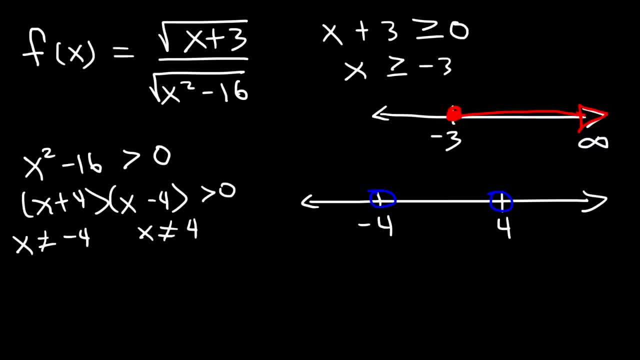 I like to do a sign test to find out which regions it's going to be negative. In this example it's going to be positive above negative 3, but negative below negative 3.. Now let's plug in some numbers. So if we plug in a 5 to check the region on the right, 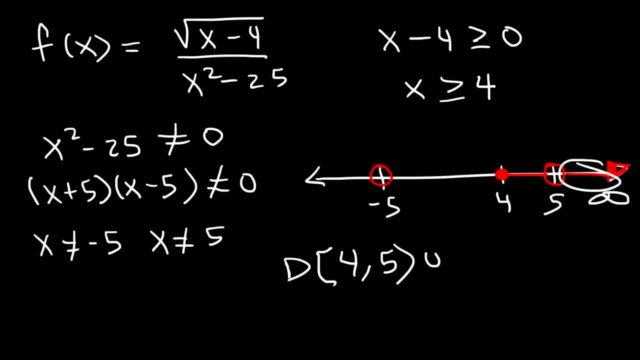 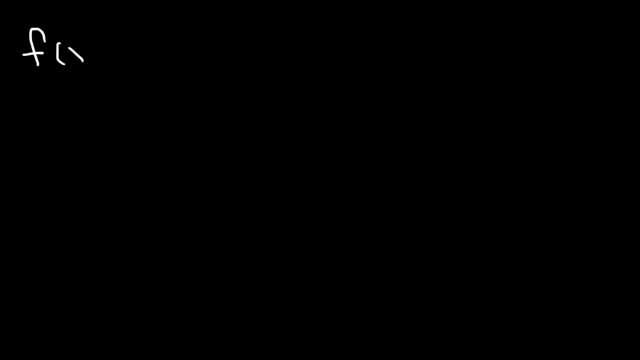 include 5.. And then union, for the second part, is going to go from 5 to infinity. So that's how you can represent the answer, Using interval notation. Now what would you do if you have a fraction that contains a square root in the numerator and also in a denominator? Try this So. 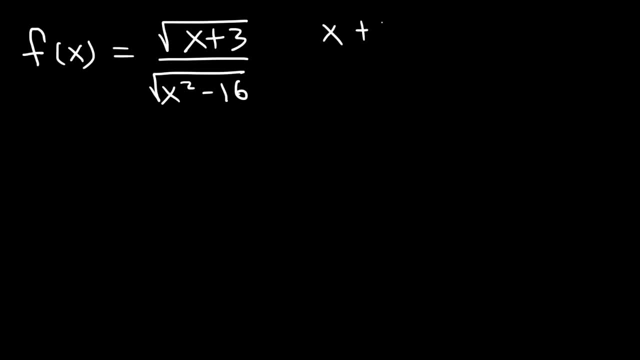 let's focus on the numerator. We know that x plus 3 is equal to or greater than 0, which means x is greater than or equal to negative 3.. So if we plot that on our number line, this is what we're going to have. 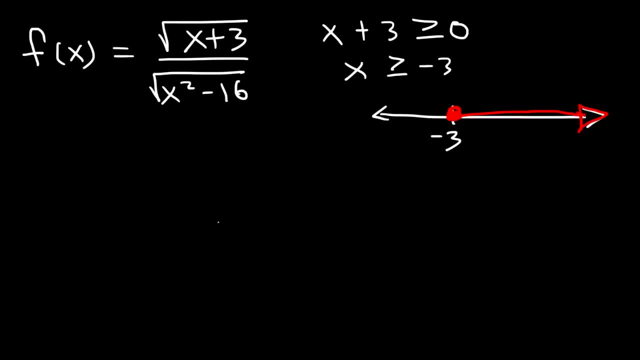 So it's from negative 3 to infinity. Now let's focus on the square root in the bottom. So we know that x squared minus 16 has to be only greater than 0, but not equal to it, because if it's on the bottom it. 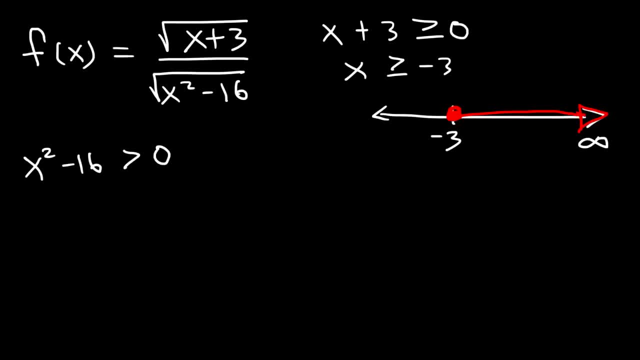 can't be 0. So if you have a square root on the top, you set it equal to and greater than 0. If it's on the bottom, simply just greater than 0. So what we need to do first is factor this expression. It's going to be x plus 4 and x minus 4.. So 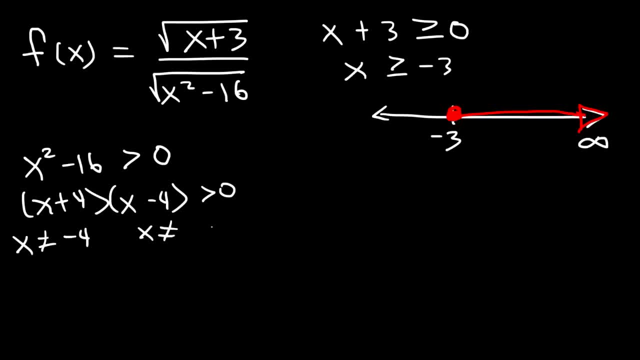 x can't be negative 4 and x can't be 4.. But it can be equal to values in between. So we're going to make a second number line. Now, the reason why I can't equal it is because we don't have the underlined symbol. It's only greater than 0, but not equal to 0.. So let's start with. 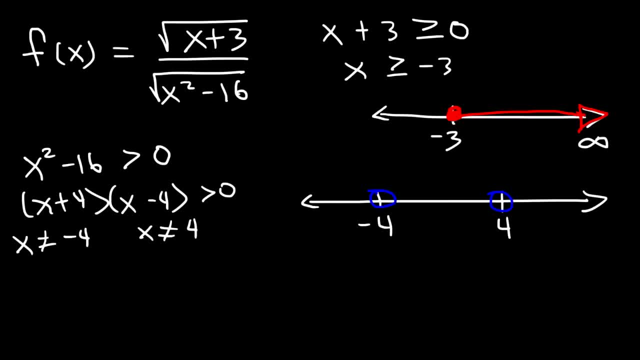 an open circle at negative 4 and 4.. Now, whenever you have like two circles on a number line due to a square root function, I like to do a sign test to find out which regions it's going to be negative. In this example, it's going to be positive. 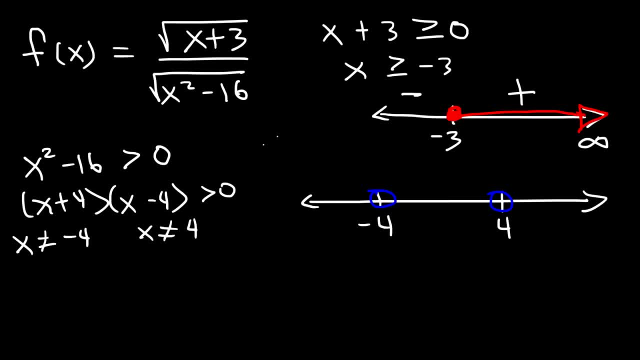 above negative 3, but negative below negative 3.. Now let's plug in some numbers. So if we plug in a 5 to check the region on the right, 5 plus 4 using this expression, that's going to be positive And 5 minus 4 is positive. So two positive numbers multiplied to each other. 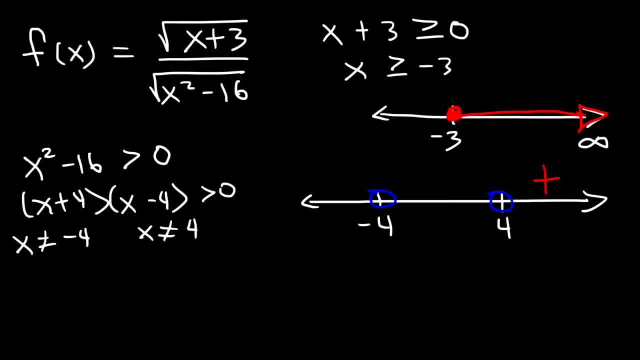 will give us a positive. If we plug in 0,, 0 plus 4 is positive, 0 minus 4 is negative. So a positive times a negative number is a negative number. And if we plug in negative 5 to check that region, negative 5 plus 4 is negative. Negative 5 minus 4 is still negative. 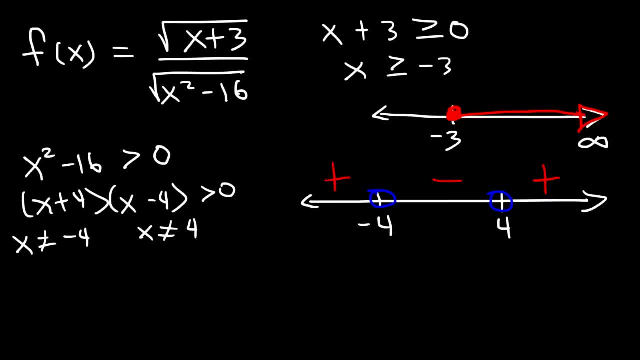 Two negative numbers will multiply and give you a positive result. So now, what should we do at this point? Now we know that we can't have any negative numbers inside a square root symbol, So it's not going to be anything between negative 4 and 4.. 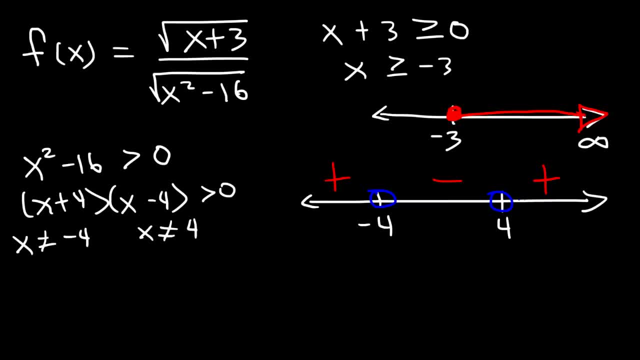 So for the square root on the bottom, x can be greater than 4 and it could be less than negative 4, but nothing in between. So now what we need to do is find the intersection of these two number lines. We've got to find out where it's true for both functions. 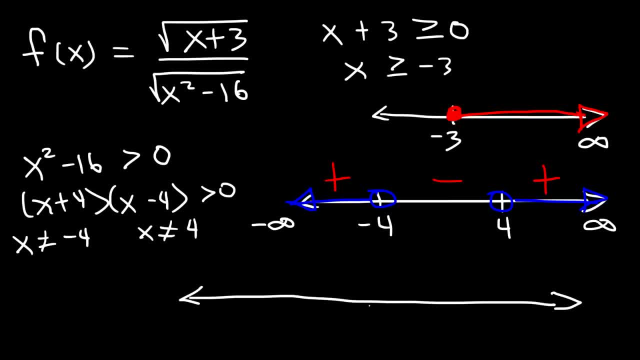 So I'm going to create a hybrid number line. So I'm going to put negative 4, negative 3, 4, and infinity, And negative infinity as well. So looking at the first one, it's not going to work if we have anything that's less than negative 3.. 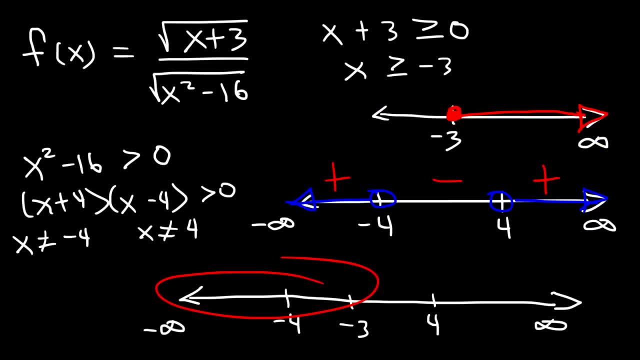 So therefore, we should have nothing on the left side. So this is going to be irrelevant, Because it's true for the second part, but it doesn't work for the first one. Now we're not going to have anything between negative 3 and 4.. 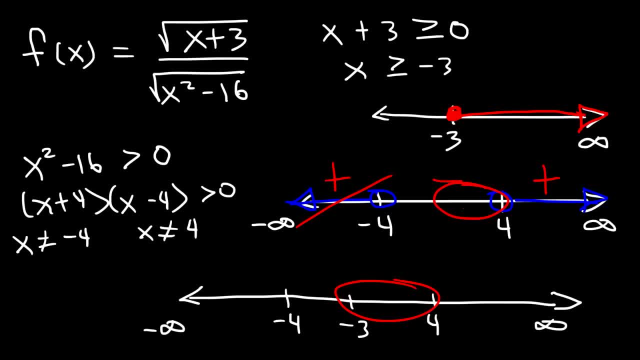 Because this is an empty region between negative 3 and 4.. Even though it works for this one, it doesn't work for the second one, So therefore the answer has to be from 4 to infinity. This region is true for both number lines. 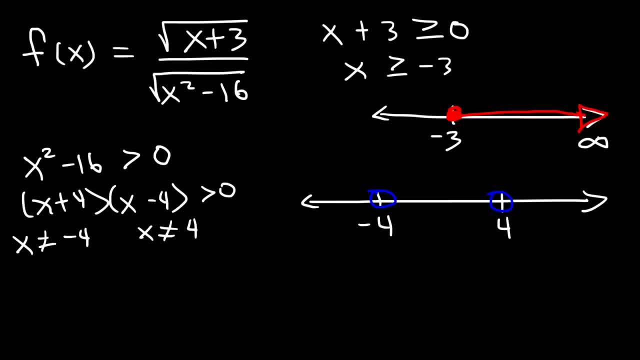 5 plus 4, using this expression, that's going to be positive And 5 minus 4 is positive. So two positive numbers multiplied to each other will give us a positive result. If we plug in 0,, 0 plus 4 is positive, 0 minus 4 is negative. 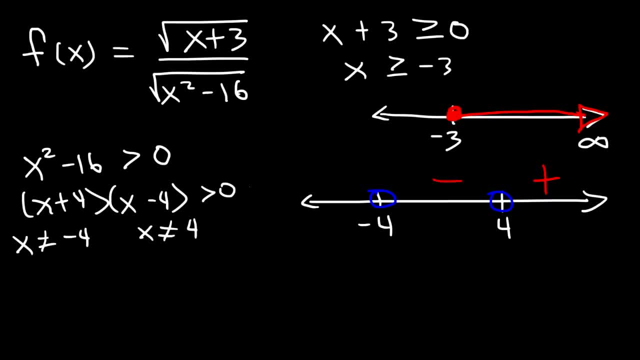 So positive times a negative number is a negative number And if we plug in negative 5 to check that region, negative 5 plus 4 is negative, negative. 5 minus 4 is positive, negative 5 minus 4 is still negative. 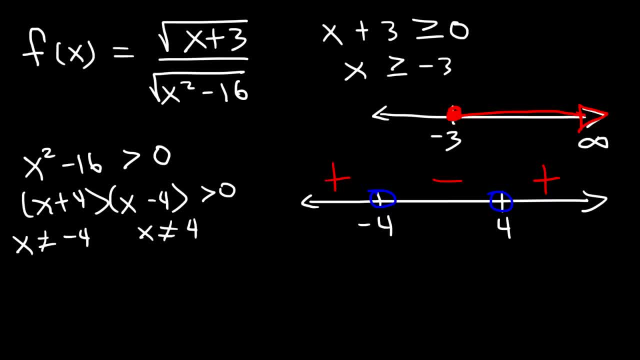 Two negative numbers will multiply and give you a positive result. So now, what should we do at this point? Now we know that we can't have any negative numbers inside a square root symbol, So it's not going to be anything between negative 4 and a 4.. 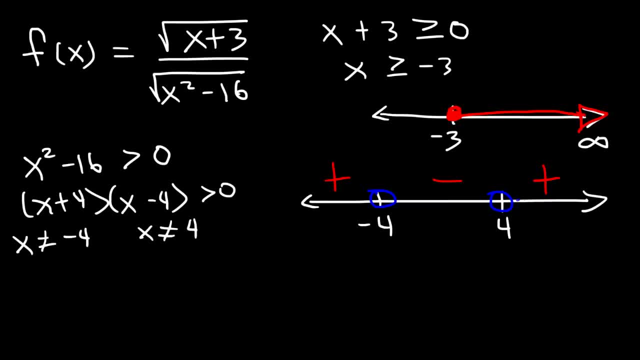 So for the square root on the bottom, x can be greater than 4, and it could be less than negative 4.. But nothing in between. So now what we need to do is find the intersection of these two number lines. We've got to find out where it's true for both functions. 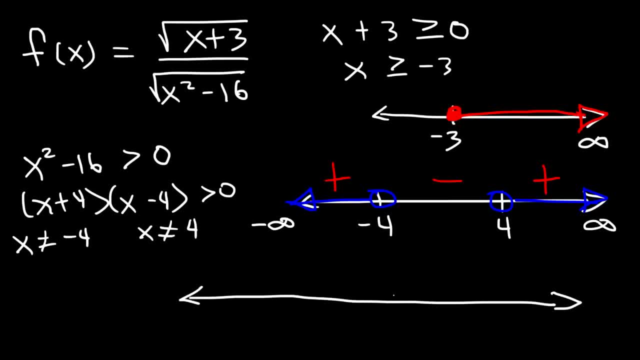 So I'm going to create a hybrid number line. So I'm going to put negative 4, negative 3, 4, and infinity, And negative infinity as well. So looking at the first one, it's not going to work if we have anything that's less than negative 3.. 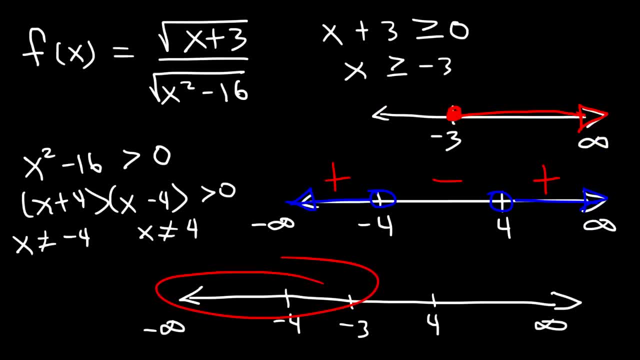 So therefore, we should have nothing on the left side. So this is going to be irrelevant, Because it's true for the second part, but it doesn't work for the first one. Now we're not going to have anything between negative 3 and 4.. 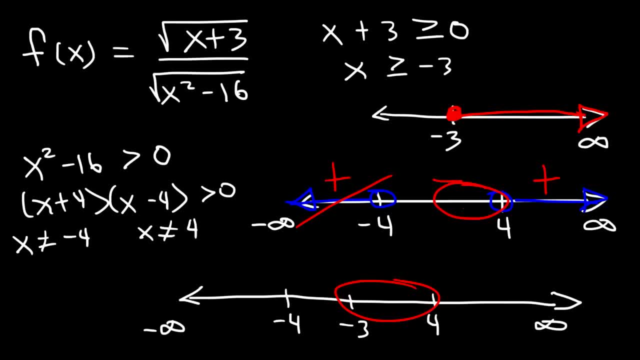 Because this is an empty region between negative 3 and 4.. Even though it works for this one, it doesn't work for the second one, So therefore the answer has to be from 4 to infinity. This region is true for both number lines. 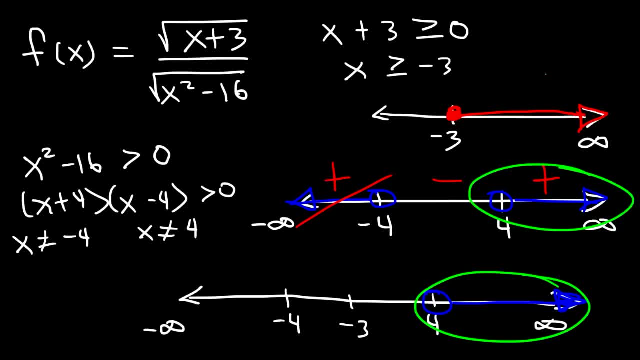 This region here applies to this number line and also this one as well, Because somewhere between negative 3 and infinity there's a 4. Now it has to be an open circle, not a closed circle. So 4 to infinity overlaps for this function on top.